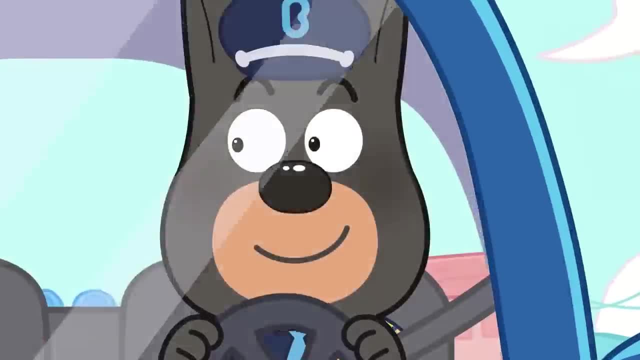 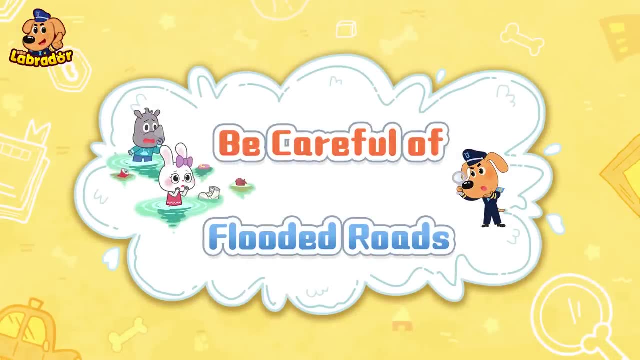 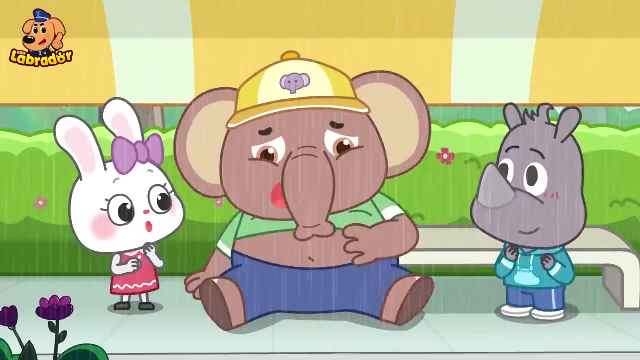 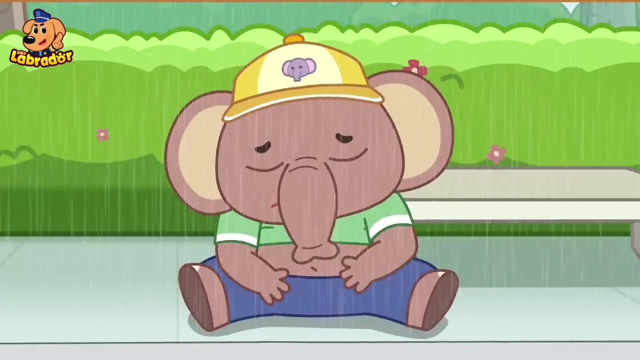 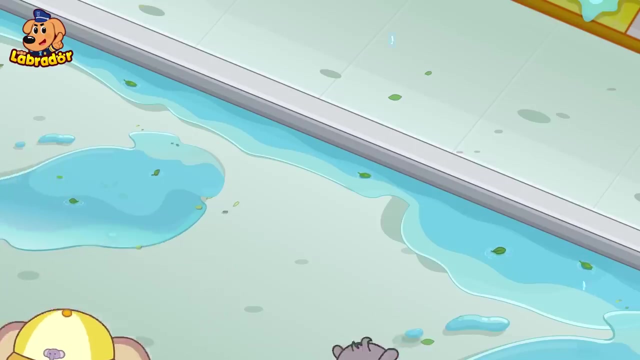 Go, Go, Go Go. Let's go. Sherry, Slap her door, Be careful of flooded roads. I'm so hungry. When will the rain stop? The rain stopped, Let's go, There's so much water. 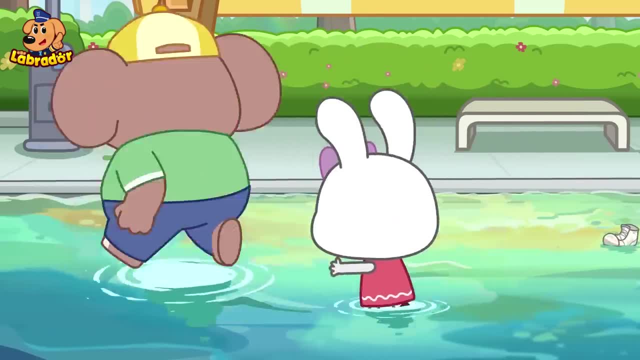 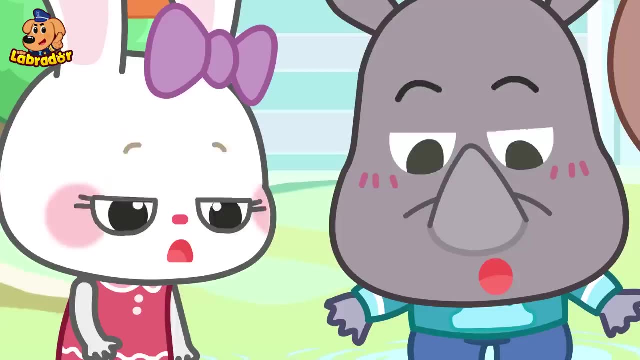 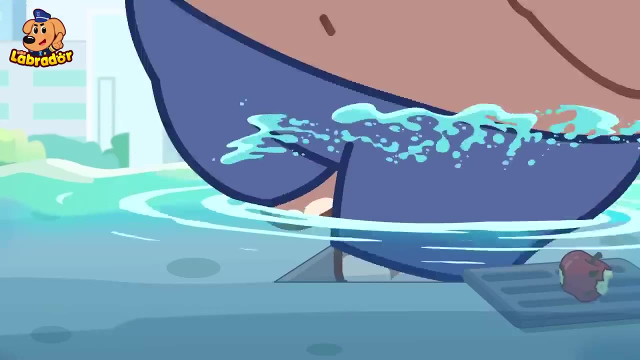 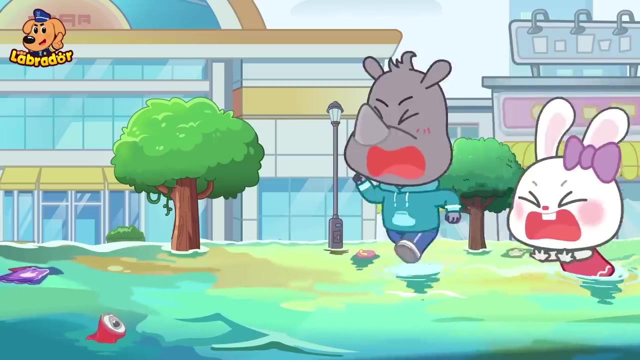 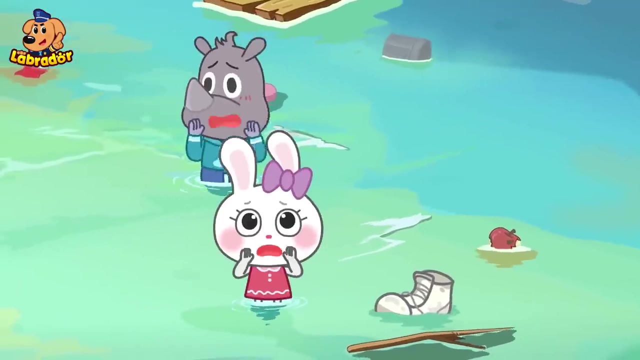 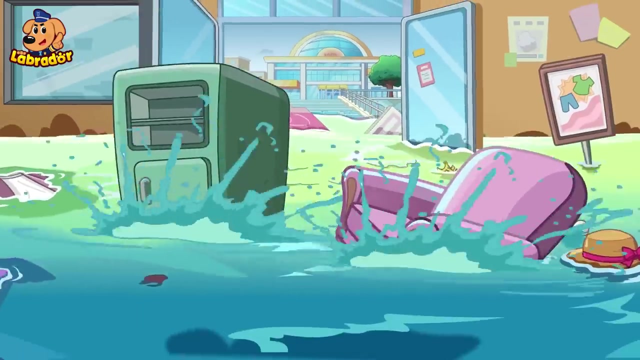 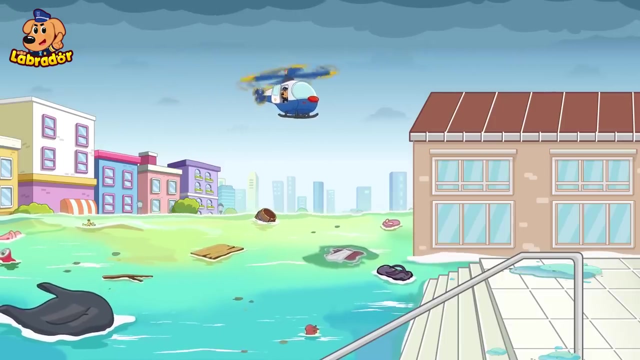 It's fine, Just walk slowly. Let's go home and eat Bugs, Bugs, Ouch. Where's Little Elephant? Little Elephant, Where are you? Help me Be careful, everyone Stay out of the water. Wait until it goes down. 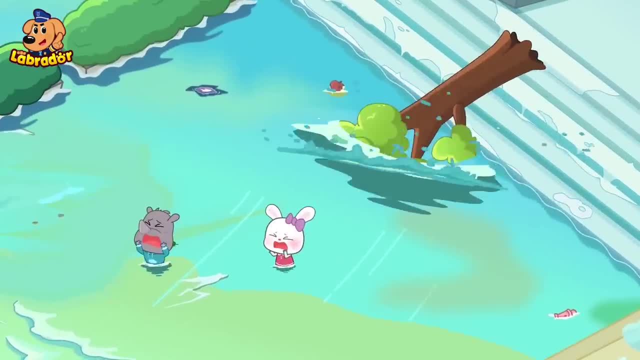 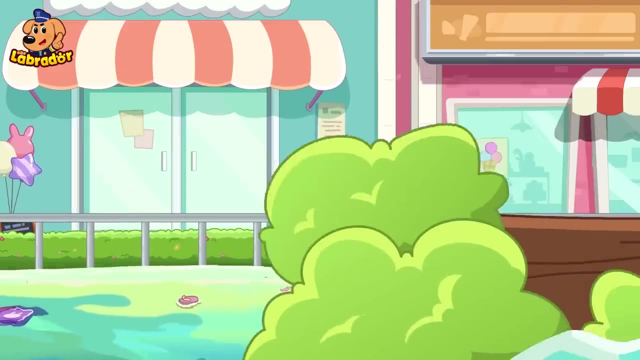 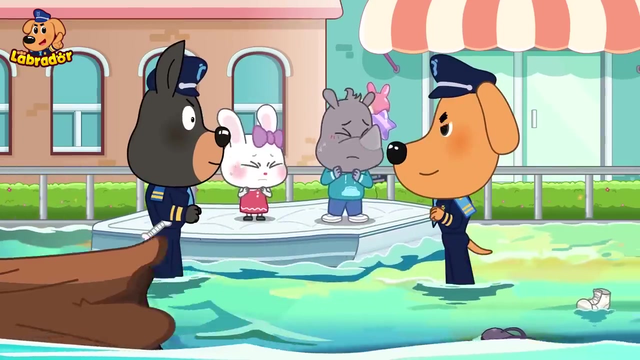 Look over there, Little Elephant, Watch out, Let's get out of here. Little Rhino, Little Rabbit, Walking on flooded roads is very dangerous. We got it, Sheriff Labrador. Little Elephant is missing. We were together and came running from over there. 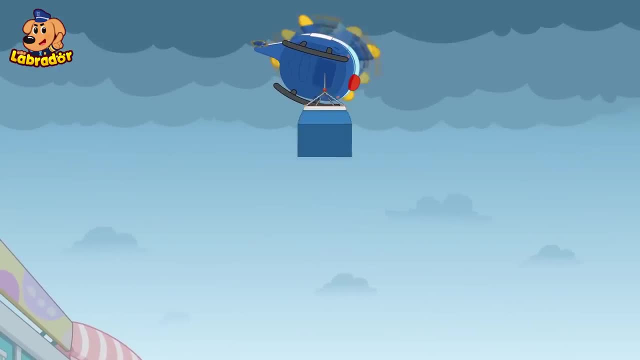 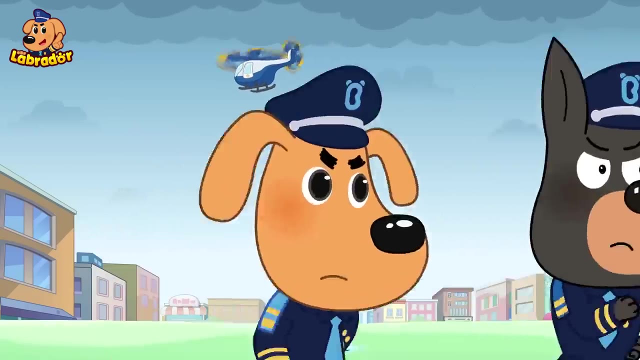 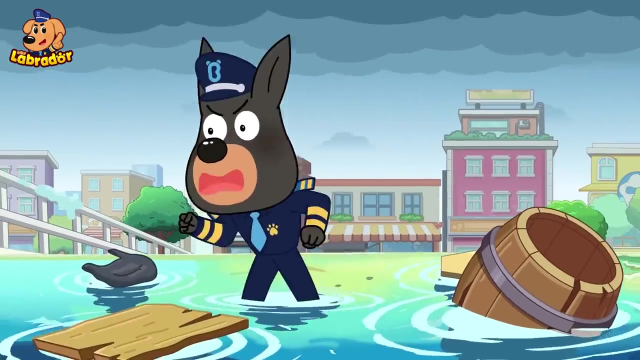 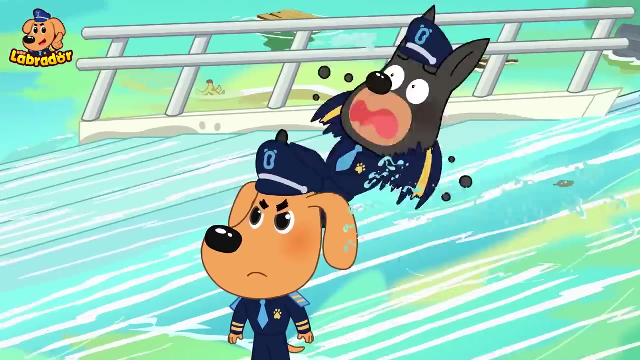 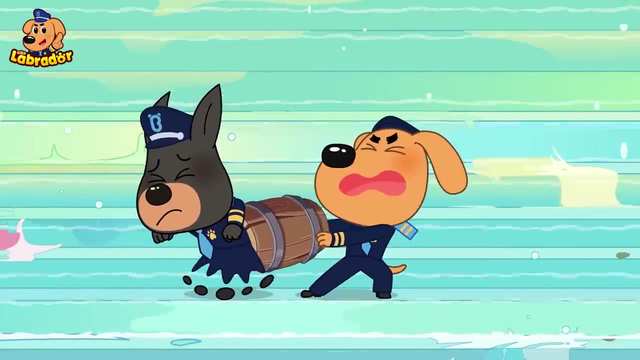 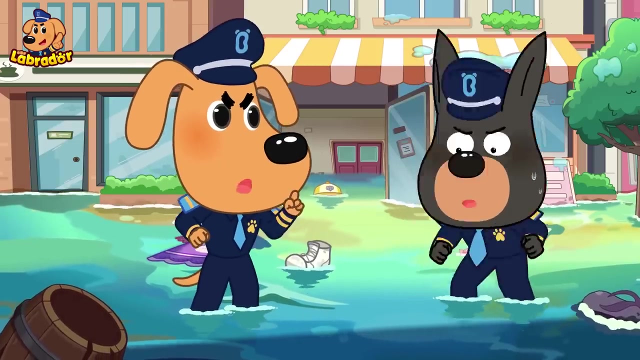 Let's go find him, Papillon, Take them to a safe place, Leave it to me, Little Elephant. Little Elephant, That's strange. Where could he be? Bugs Ouch Harris, stop SBS. Toby, You can't see what's under your feet on a flooded road, so be careful. 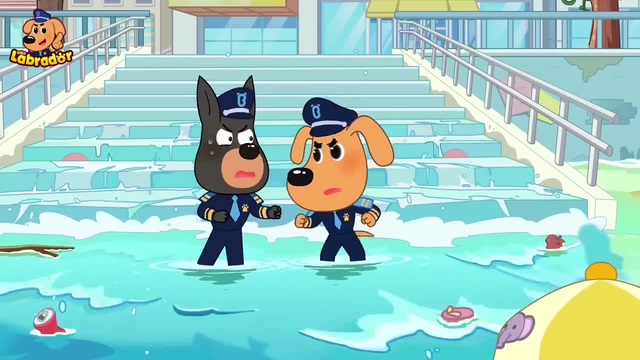 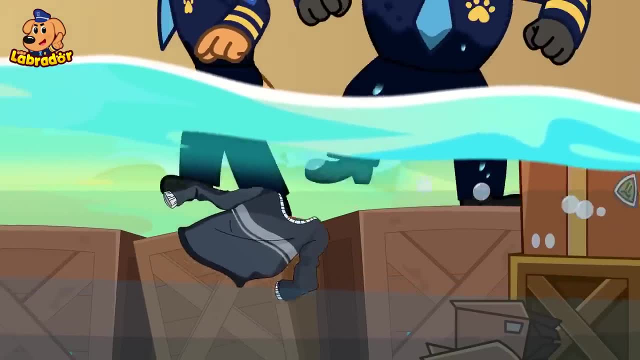 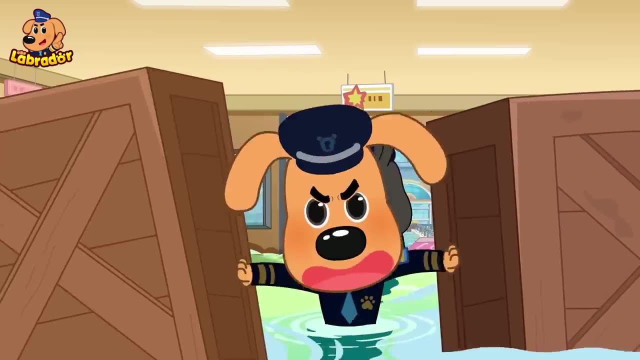 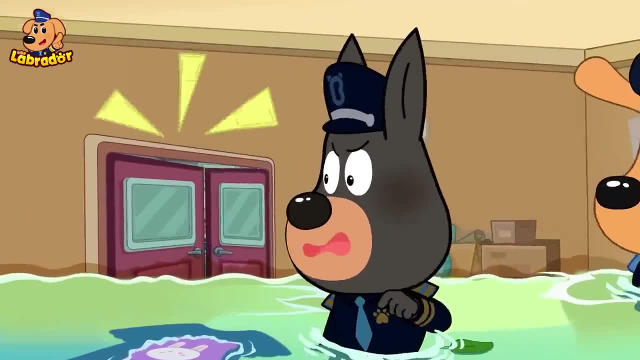 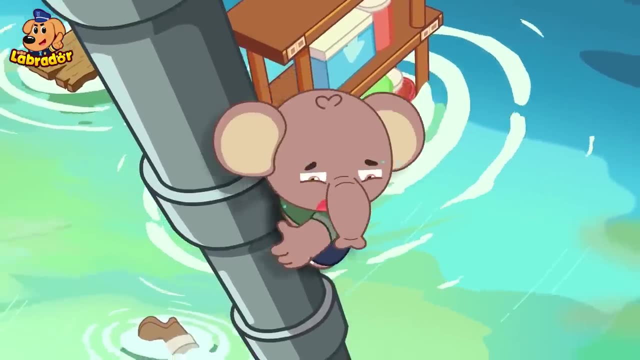 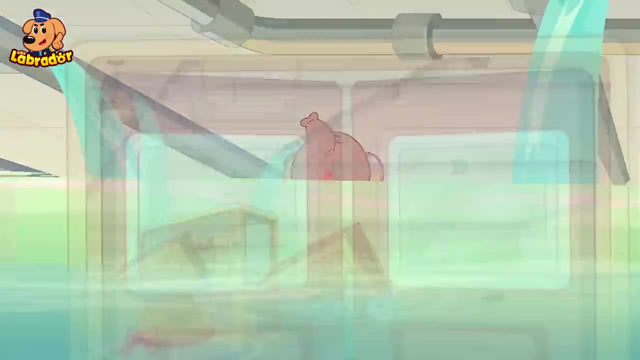 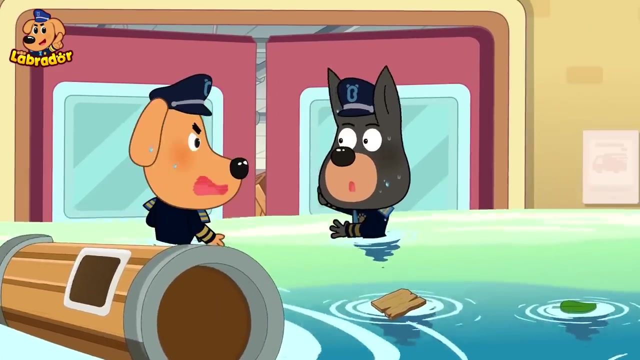 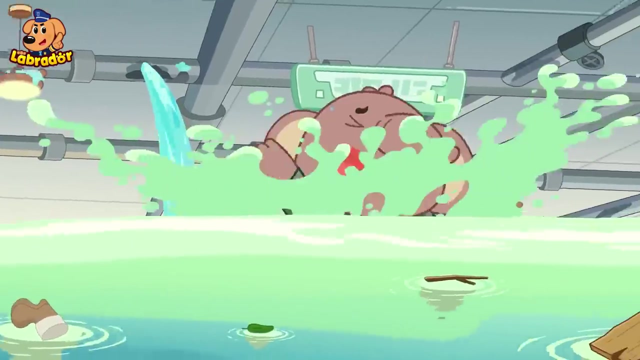 It's just a big fish. Help me, What do I do? The water's rising. Ah, Ouch, Somebody help me. Little elephant is inside. It's blocked. Toby, I have an idea. Go, Little elephant, Help, Help me. 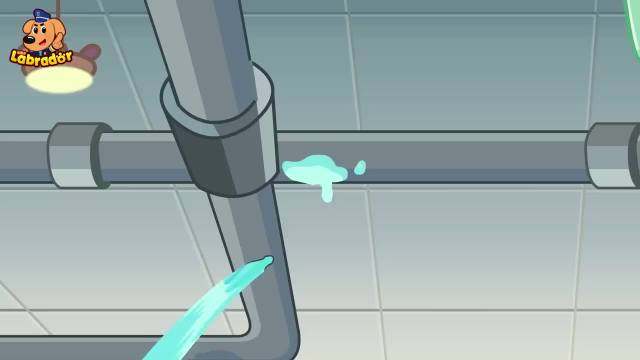 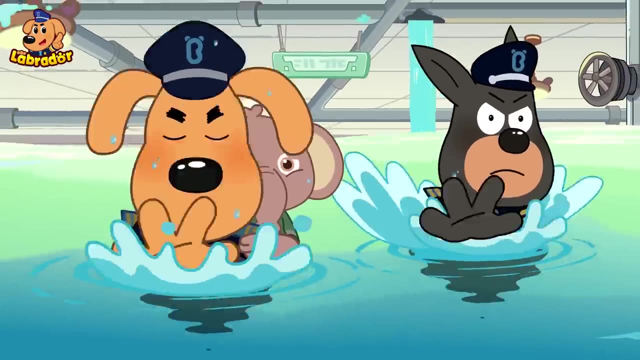 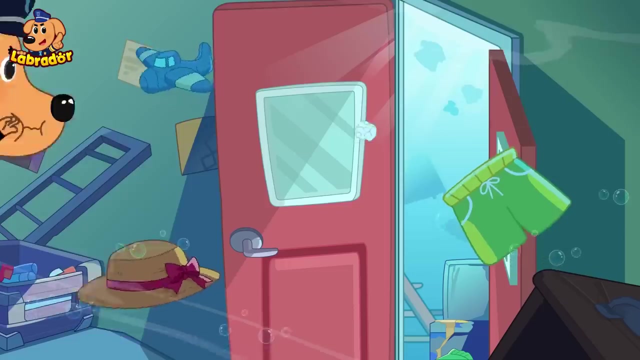 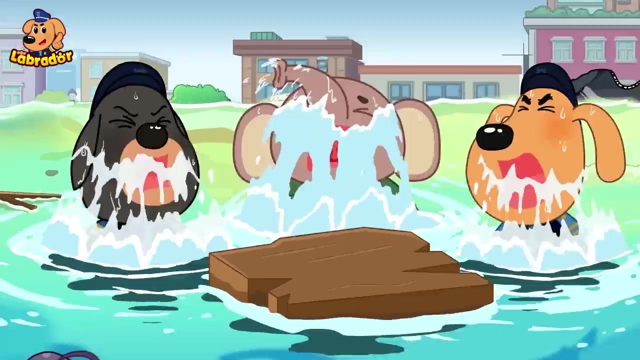 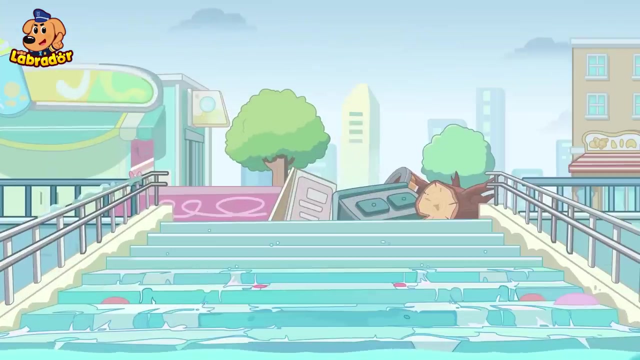 Sheriff Labrador, Let's go. Let's get out of here. The water is rising. This place will soon be flooded. We have to dive in. Everyone, hold your breath. We made it out, Oh no, The water is rising. 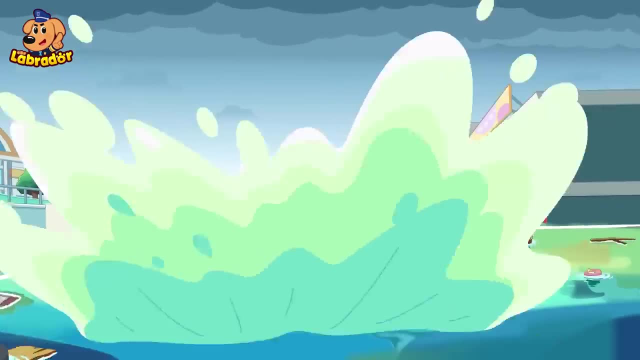 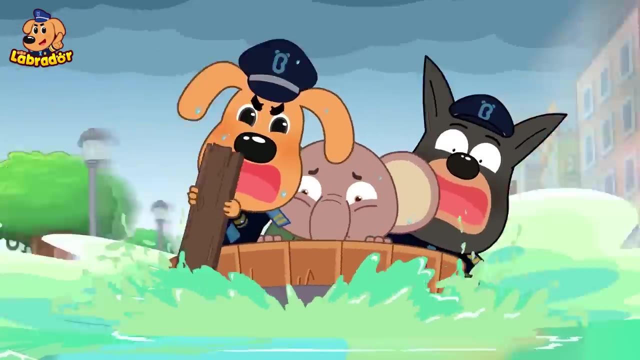 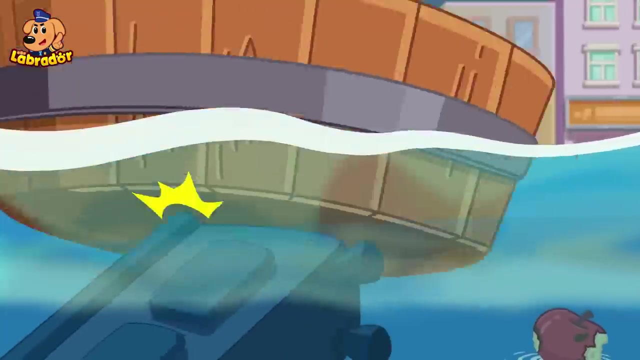 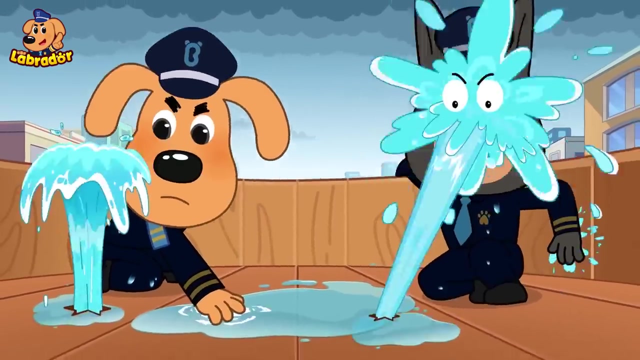 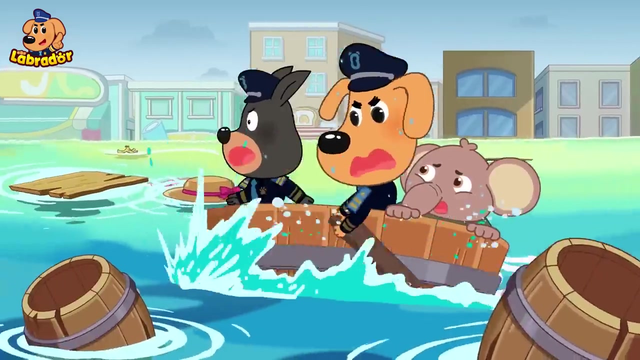 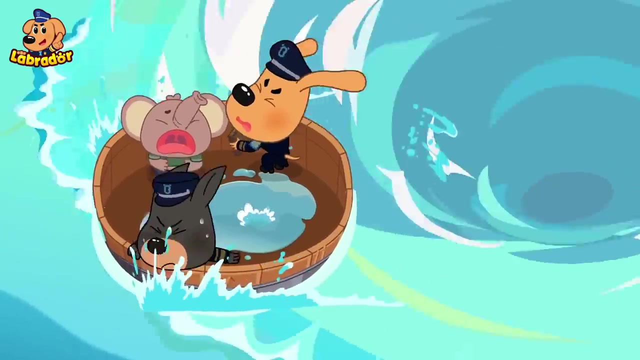 The water is rising over here. Hurry, Jump into that basin Paddle- Oh no, It's leaking. What's that? Oh no, It's a whirlpool. Roll back now. I can't get out of here. Help. 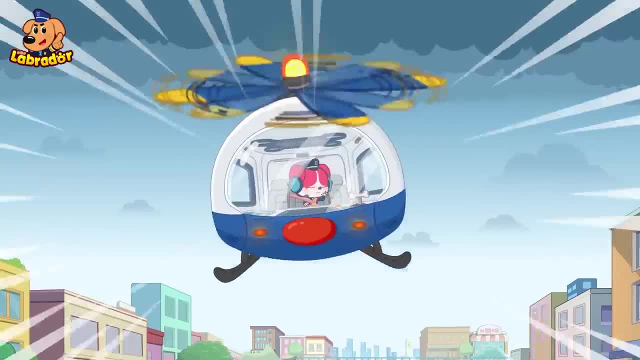 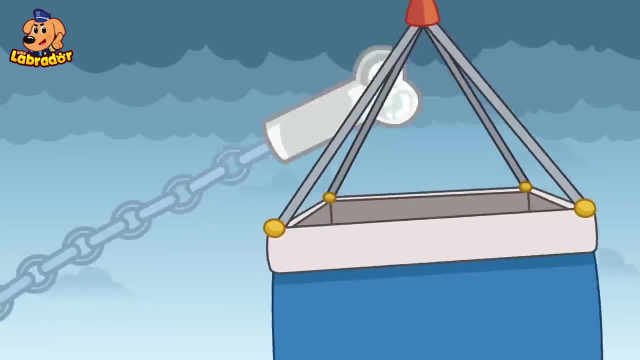 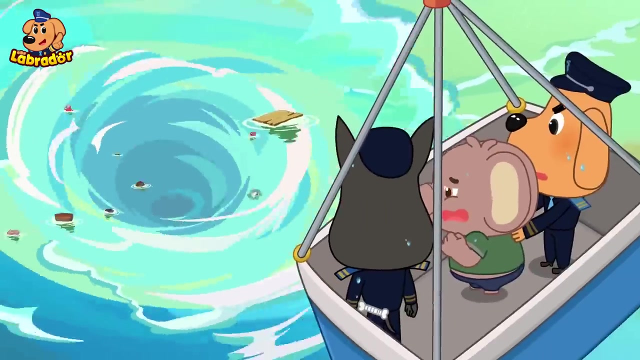 Help Coming. We're out of here. I can't get out. I'm all wet. Get on the rescue basket. What a relief. Oh no, Toby, I can't get out of here. Oh no, Oh no, Oh no.